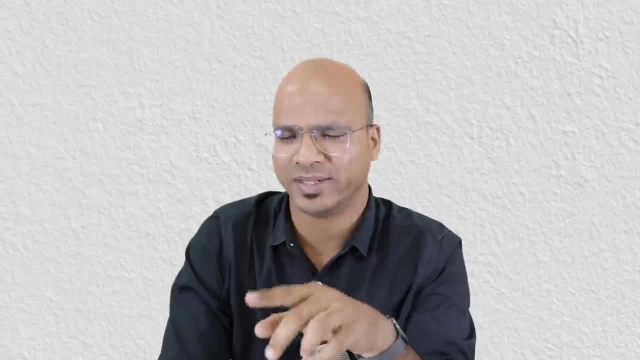 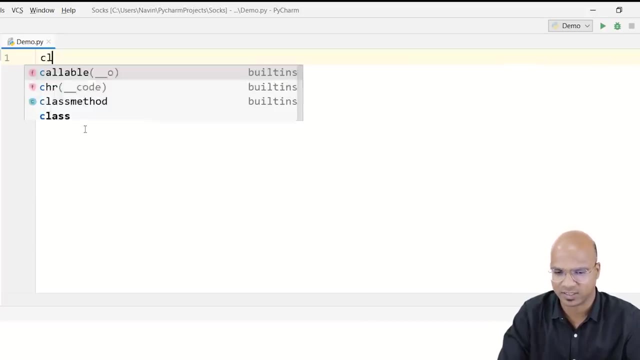 is abstract class and why do we need it? So we'll start with what and then we'll discuss why do we need it. Okay, So what is abstract class? So basically, let's create a class here and we can create a class name, let's say computer, And of course computer can have multiple methods or 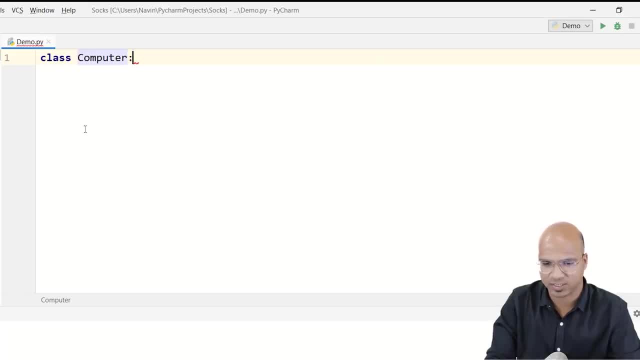 multiple functions here And I will say: okay, that's a computer class, And in this class I can create some methods. Now, how do we create methods? It's very simple, We say dev And then let's create a method which is, let's say, process. It's a computer process, right? And 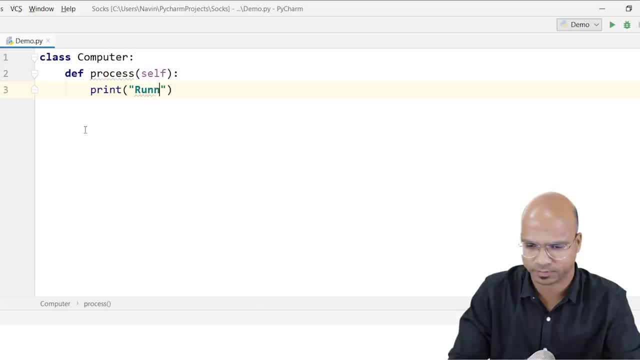 then I can print here, I can say: running, Nothing fancy, Let's keep it simple. and we say: running here. So that's how we create a class and that's how you create a method. Now, how do you make a method? So a method has a name, A method has parameters which it accepts, or arguments, And 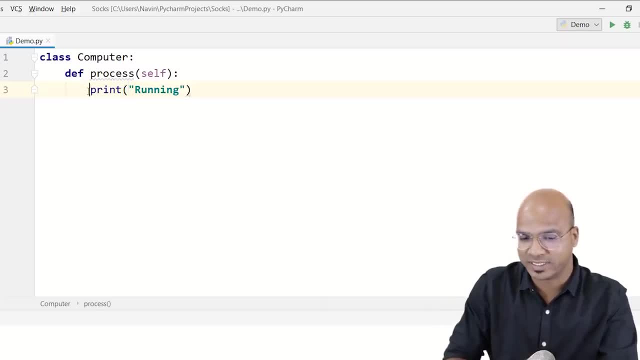 then method also has a body. So this body here, this print statement is a body, So this body here, right? So this body can have multiple statements. We can say: we can do some processing there, We can take values, We can take variables and we can do some operations. But then just to keep it simple, 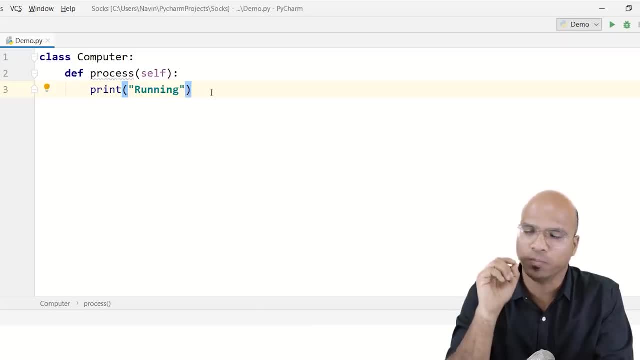 this method has only one statement. Now, whenever your method has a body, it's a normal method. So, and normal methods are the normal classes. But what if I don't want to mention anything inside this method? I want to keep it blank. I just want to declare this method. Now, when you declare it. 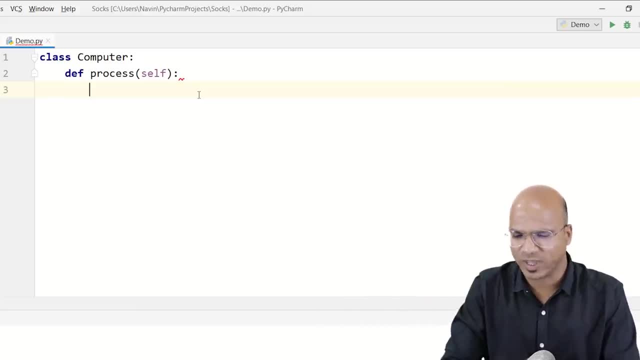 simply means that it doesn't have a body right. So I want to keep it blank. I just want to declare this method Now. when you declare it, it simply means that it doesn't have a body right Now. the way you can declare a method is by saying pass. So when you say pass, 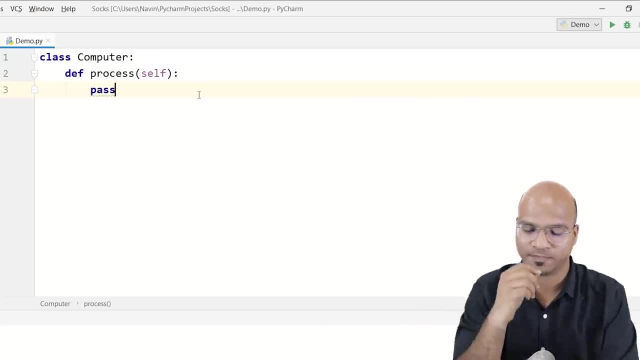 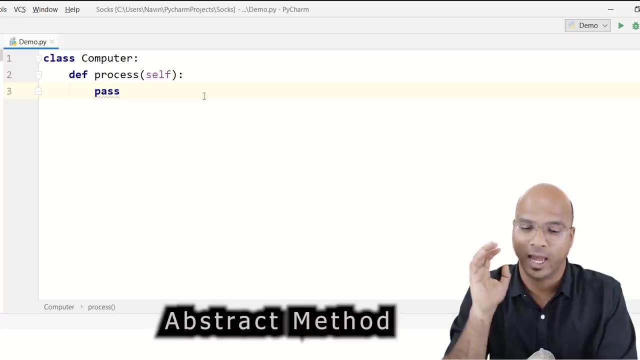 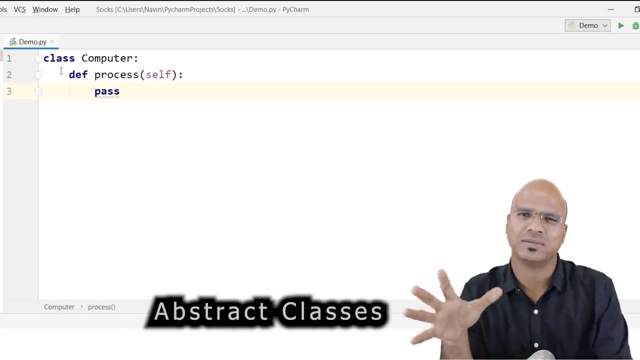 it simply means I don't have anything inside this method. Now, this method which only has a declaration but not a definition, we call them as abstract methods. right, And then a class which will have abstract methods is called abstract classes. But then this type of concept is there. 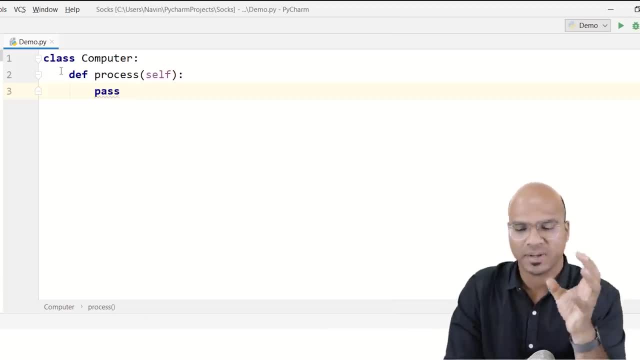 from another language as well. It is in Java, in C, sharp. But then Python is a bit different, right? Because Python by default does not support abstract classes. Now, if you want to make an abstract class and do something, and that something is because there is- 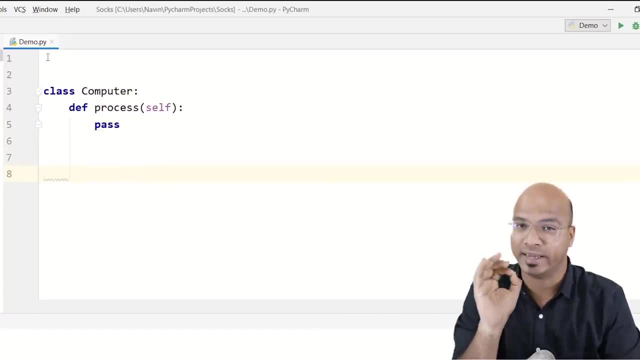 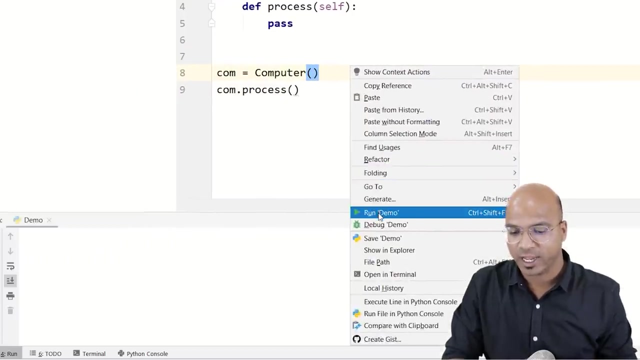 one more definition. there is one more thing for abstract class. you cannot create a object of it. Example: if I try to get object of computer here and okay, And if I say comprocess, you can see there is no error, at least when I am typing this, If I don't have this code. 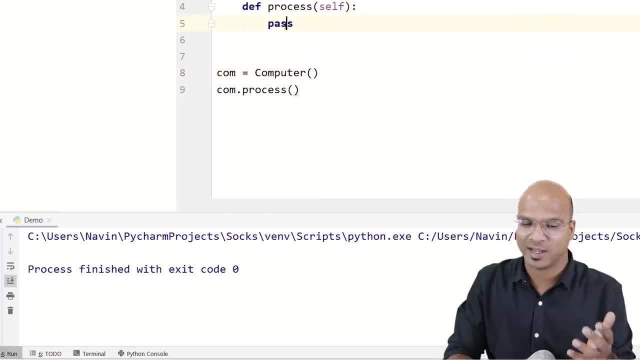 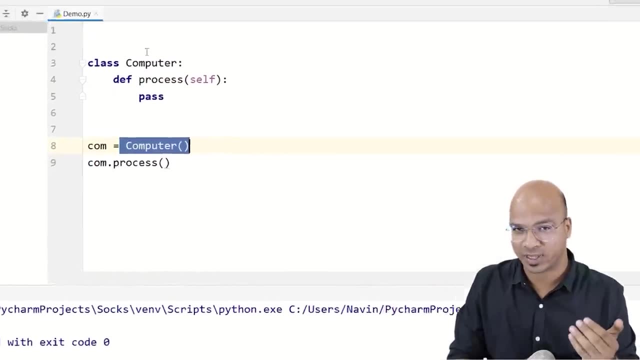 it perfectly works. There is no output, of course, because they are saying pass. The thing is, we are are able to get this object because this is not an abstract class. yet how do you make it abstract class? and for that you have to import a module. so which module you have to import? so you have to. 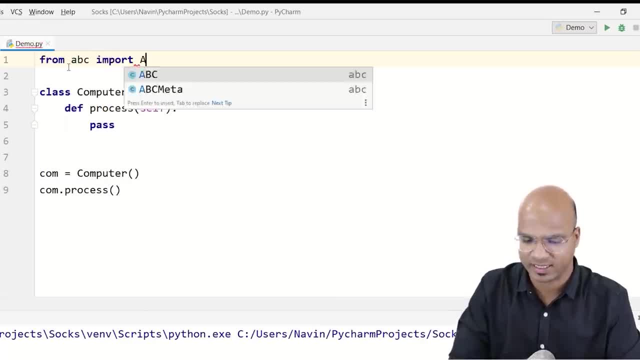 import abc and in this you have to import only two things. one is abc, which is abstract base classes, and you need to also import the method abstract method. so this will make this class as a subclass of abc, so that this also becomes abstract class. so now this is abstract class and then this method. 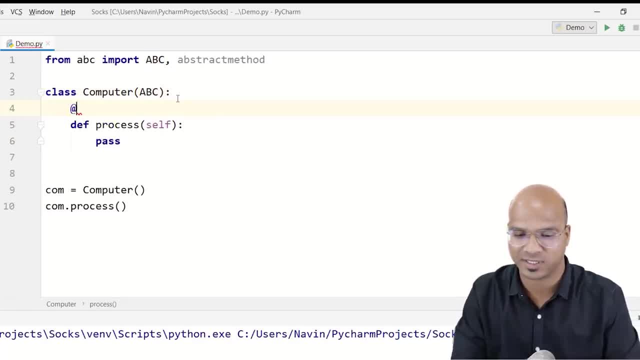 has to be abstract method, so we'll say so. we'll use a decorator here, which is, at the rate, abstract method. now, using decorator, you can mention: hey, this process is a method which is abstract, so you're talking to your compiler about it. now, once you do this, and if you run this code, 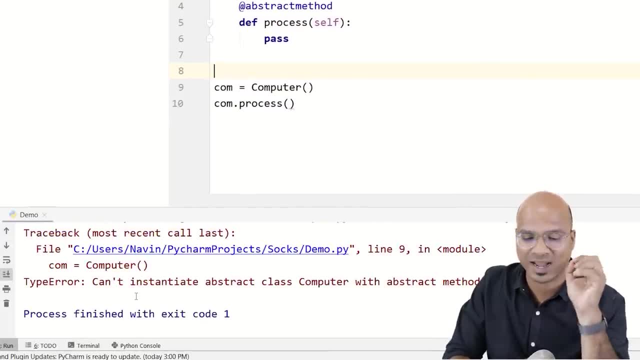 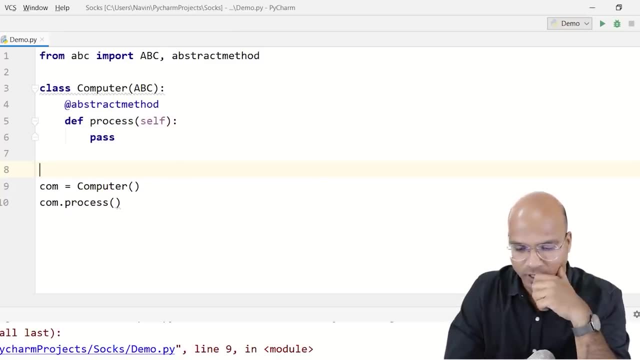 now you can see we got an error. it simply says: can't instantiate abstract class. that's important. now, if you make a class abstract, you can't create object of it because because we have a method which is, which is not defined. now, that's something you have to remember. now we can. 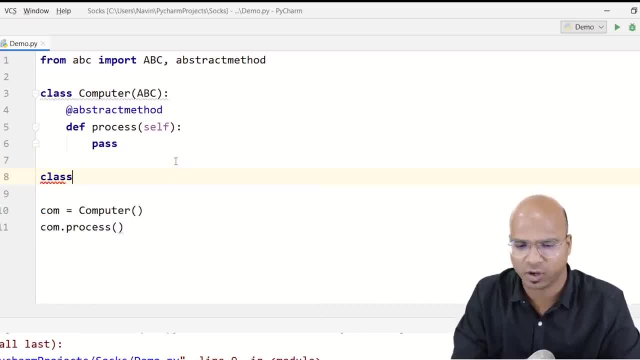 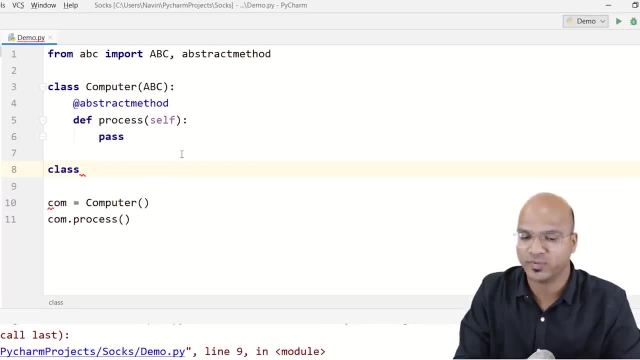 create multiple classes here, example, i can create one more class. of course i can't get object of a computer because it's an abstract class and has a method which is undefined, which is declared. so what we can do is we can create a new class which is laptop, because when you say computer, computer, 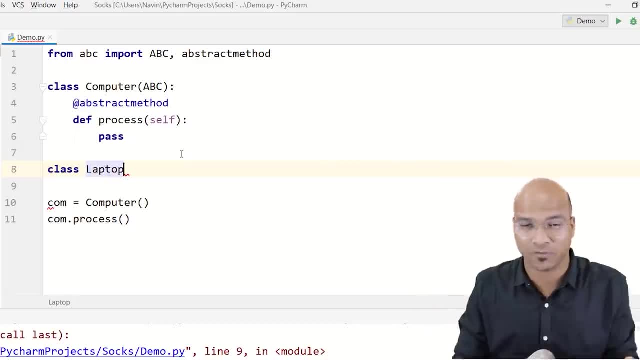 is just a fancy term, right, because we don't buy computers, we buy laptop, we buy dexter, we buy phones. so this laptop is actually a subclass of a computer. and then here i can define that method. but what happens if i don't define methods? in this case, if i try to create? 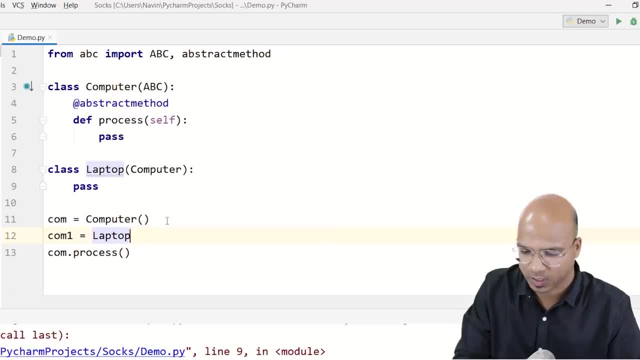 object of laptop. so you can see, if i say laptop, what do you think will it work? so before continuing, you can pause the video and you can answer in the comment section: what do you think will it work or not? because this time i'm not getting object of computer, i'm getting object of laptop. will it work? 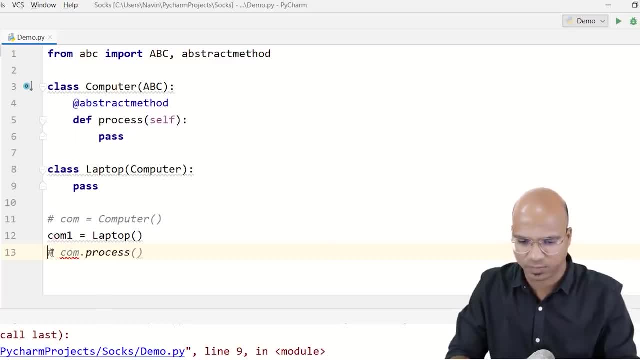 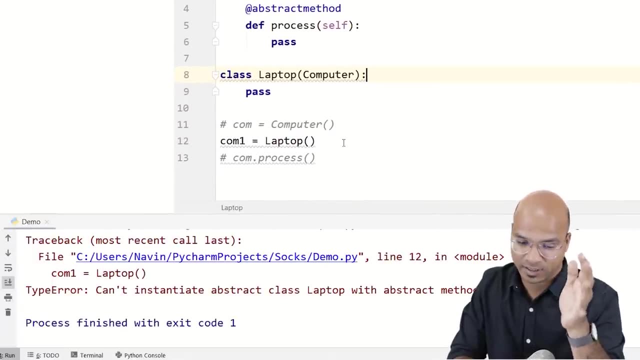 and then i'm: let's say: i'm not calling anything, it just i'm creating the object on site now and let's run. i hope you have answered and you can see we are getting error. the error is instantiate abstract class laptop with abstract methods process. now that that's a thing. laptop is. 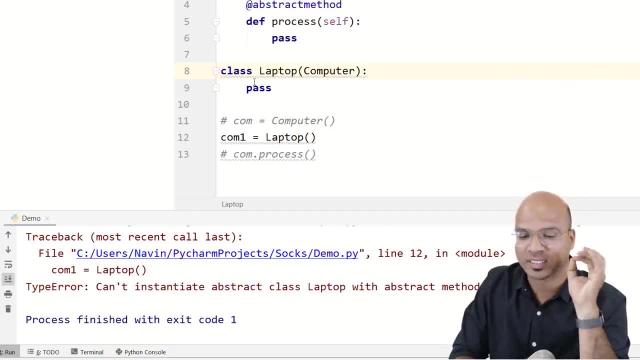 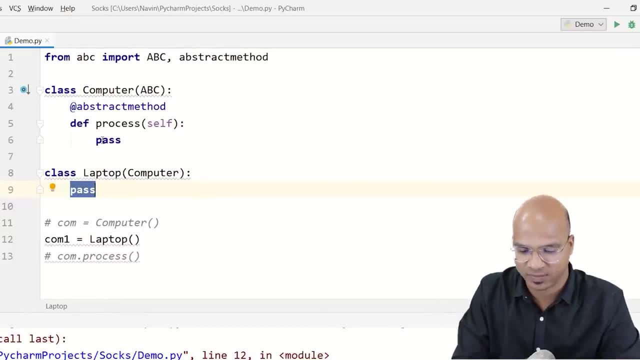 inheriting computer in which you have abstract method. so it is compulsion for you to define that method. otherwise even this class, which is laptop, is abstract class. so in this case i will simply say def and i will define the method, and then i will say process. 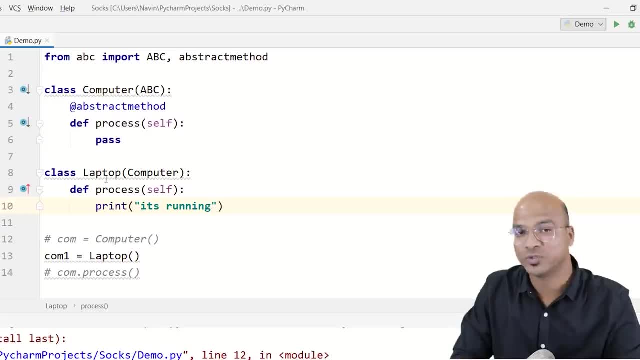 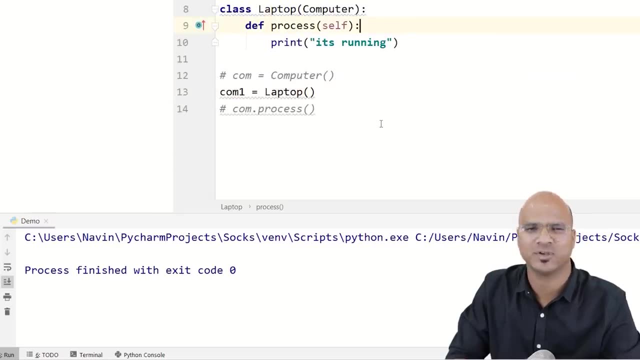 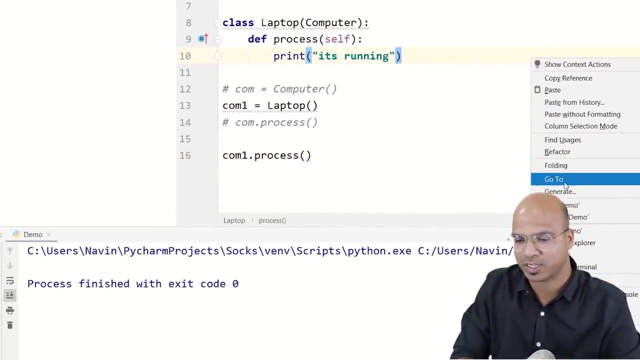 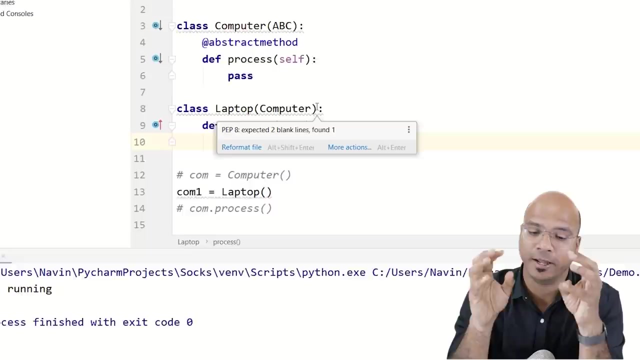 it's running, that's it, nothing fancy. will this work? let's try now, because now i'm defining that. So if I say run and it worked, It's just that I'm not calling this process. That's why you don't have any output. You can do that. We can say comp1.process. At least I can see some output in the console And we got the output. That's great. So this is working. So you can see, we can create a class and that class will implement all the methods. That's important. 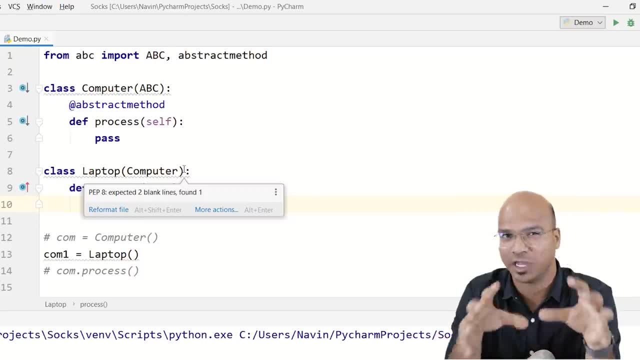 And if you fail to implement all the methods, all the abstract methods, you will get an error. Now, this is what abstract class is. Abstract class will have at least one abstract method. That's important. Right, Okay, Now, this is good. This is something you will say: hey, okay, this is a concept and it is working, But what's the use of this? Now, think about this. Whatever concept you have learned till now, everything makes sense. Right, You know how to use loops, You know what these variables are, And we can use them in the real life. 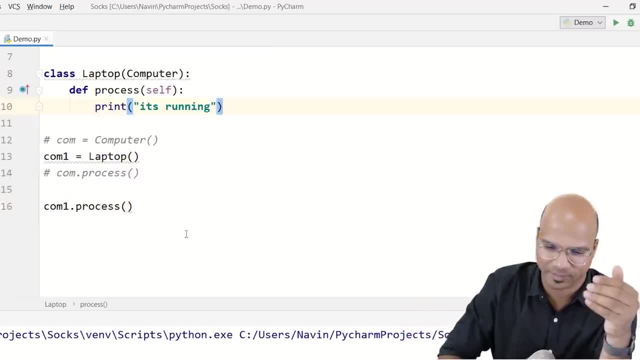 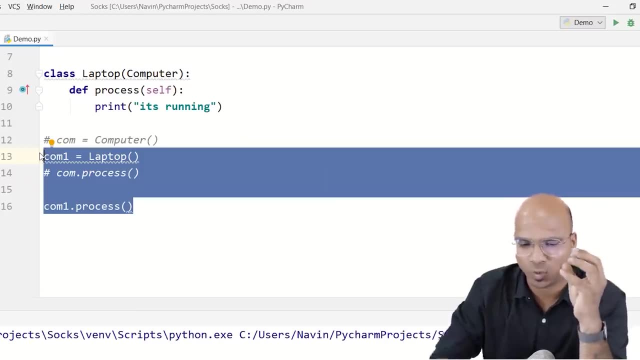 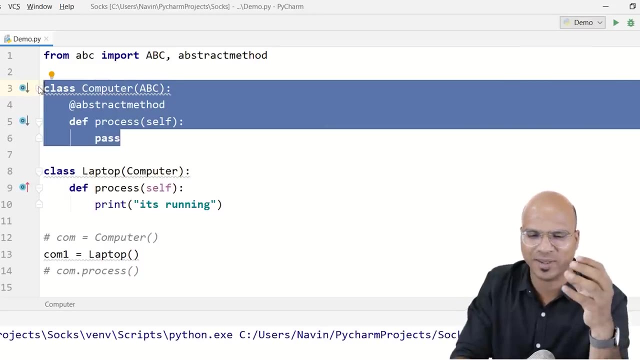 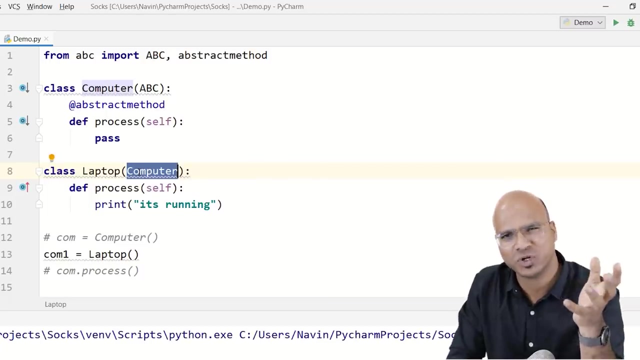 But what about abstract class? Because if you look at these two statements, we are calling a method, which is process, And then this process is getting called from laptop. So what is important here is a laptop class. What do you think is the use of this computer class Anyway? so even if I remove that, it will not make any difference. Right, I can simply remove this class, I can remove this computer as extends and it will surely works. See, this thing makes sense only when your class computer has some extra methods. 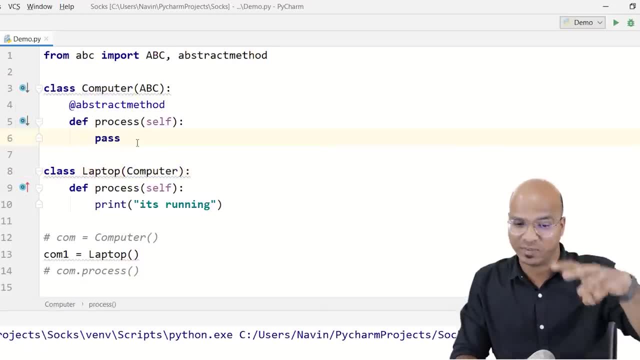 Right. Which laptops needs Right? What if you have two methods here or three methods here and laptop is taking those methods directly, Then it makes sense to use a computer. But what if your class only has abstract methods? Does it make any sense? 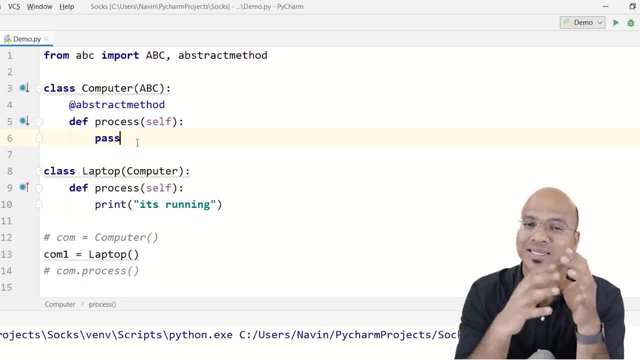 So the answer is yes. it makes sense only when you are designing an application in a oops way. So basically, when you follow the concept of object-oriented programming, you have to follow some patterns, And one of the pattern is: let's say, if you have a laptop, you have to follow some patterns. 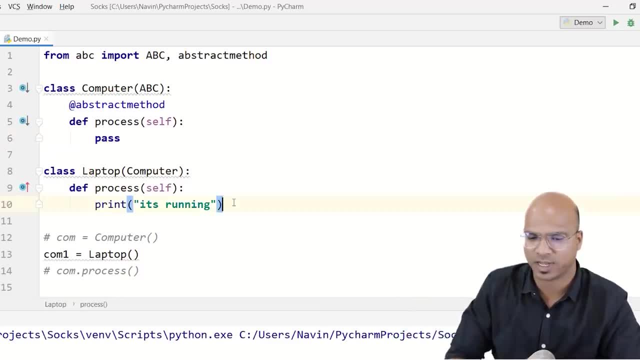 So so let me give you a classic example from a robot Who would do that. You know, if your IDE is planted inside a program and you all touches device like this one, you have to look at words, because this звон only overwrite. 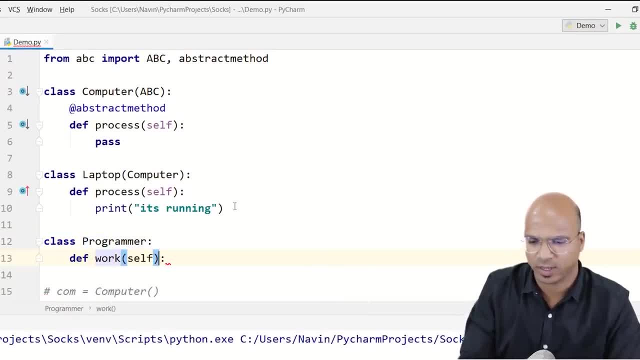 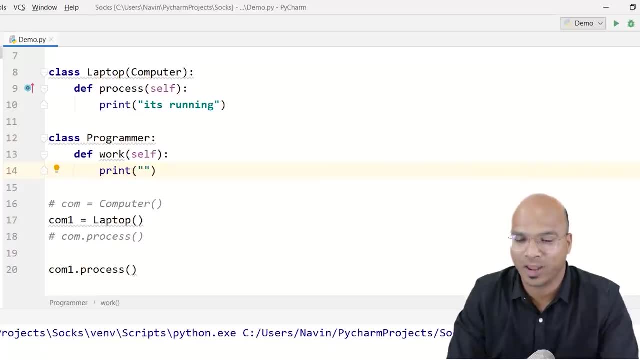 Right. So just because these variables have ahes to do that your web ultimately doesn't need a common latency, Does it mean that when I have other programs they all run in the same way, but using only one method or in the same format? 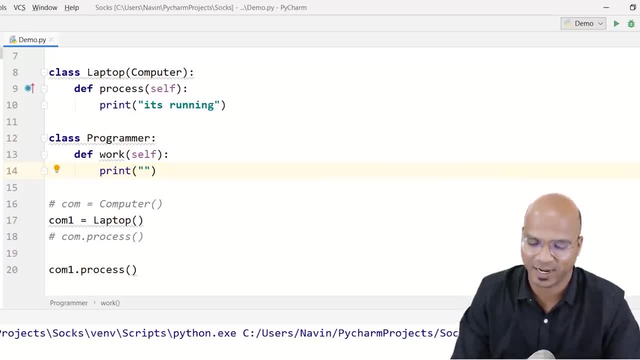 Yes, So it's good to know. in a robot鏈 can work like that. That's why they're called dynamiceria Plus. it can help you to load whatever words you want to load. So if you have Function Right. 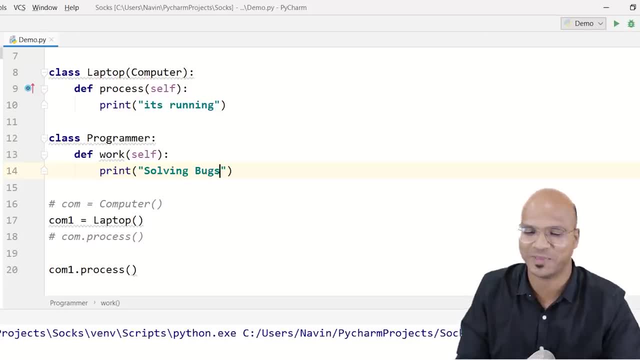 Wow, Yeah, Right, So this is working. Yeah, do we solve bugs? that's like that. that's why we spend maximum time, right? okay, so as a programmer, we do that, and let me create an object of a programmer here. i'll say: prog1- equal true. 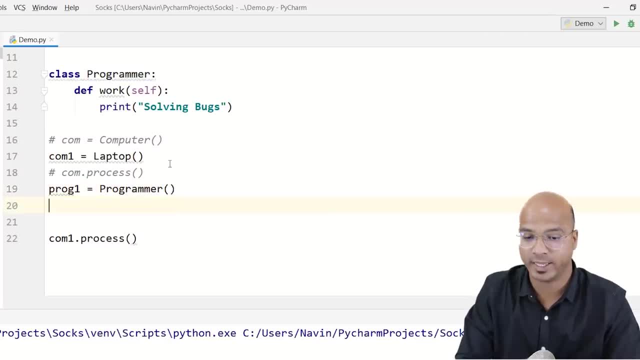 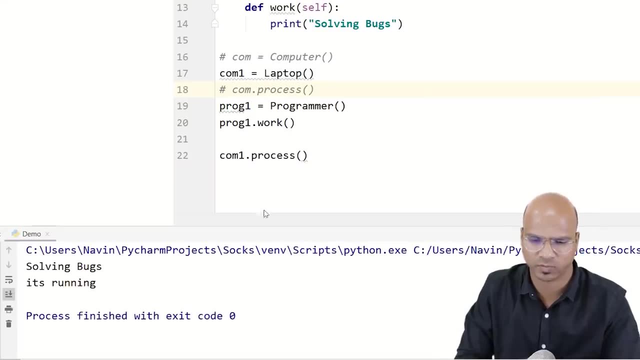 programmer and once we got the object, i can simply say: prog1, dot, work, and of course this should print something. this would. they should print solving bugs, and it should. it will print it's running, because that's what we are doing in process now. what's important is, as a programmer, you need a 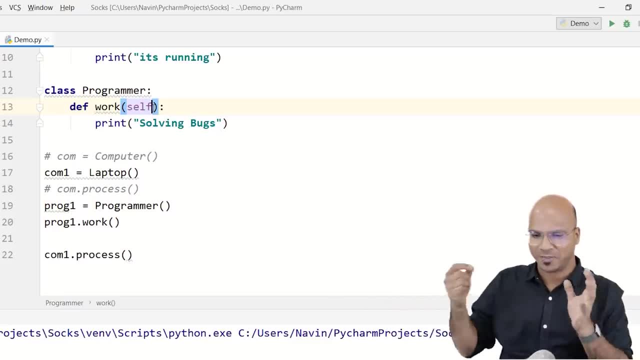 machine to work with right. of course you can't work on paper, right programmer, write codes on on laptop, on mobile phone, on on desktop. so of course you, you need a computer here. now, what do you think? what type of object i will pass here? will it be a type of laptop? will it be a type of? 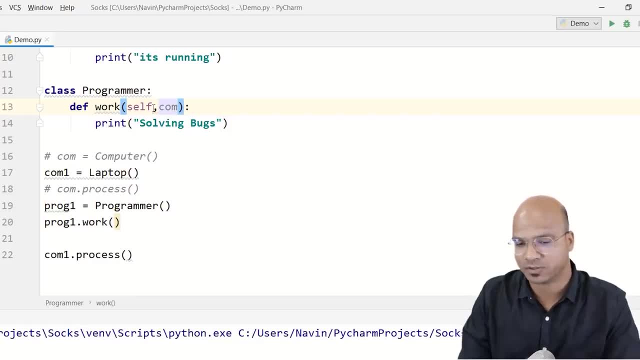 computer. so what we can do is let me pass a computer type, so we just i will say: com now. this com can be anything. this can be a laptop, this can be a desktop, right, or it can be anything. it can be a mobile phone or it can be a board whiteboard. oh, will that work now? 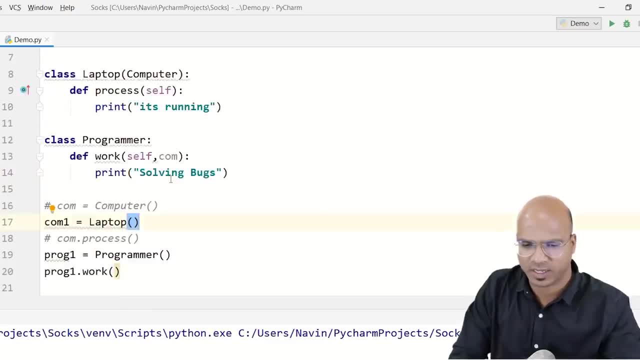 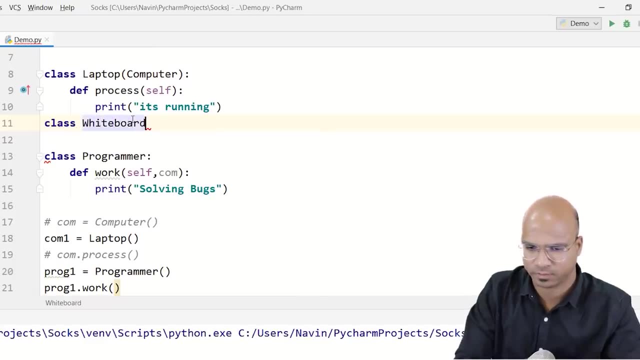 can i say, can i pass an object of a whiteboard here? so let me create a class whiteboard. i mean just to see if that works. i will say whiteboard, and of course whiteboard will have certain methods. of course it will. it will not have a. 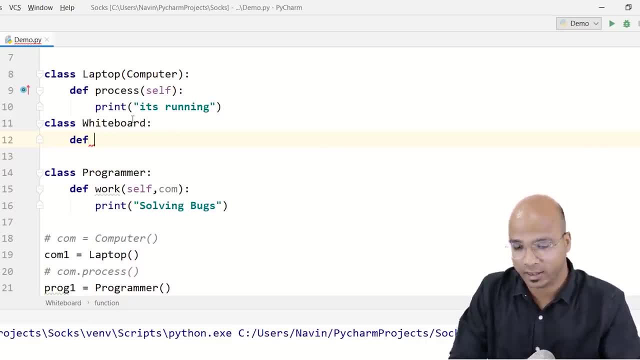 method which is process, but at least we can have a method like: and then there's one more thing in this print i will also do something with: with com. i will say com, dot, process, right. and in this whiteboard i have a method which is, let's say, write: that's what we do on boards, right? and then here i will. 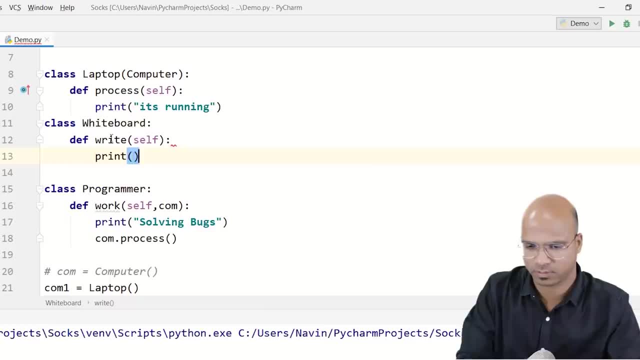 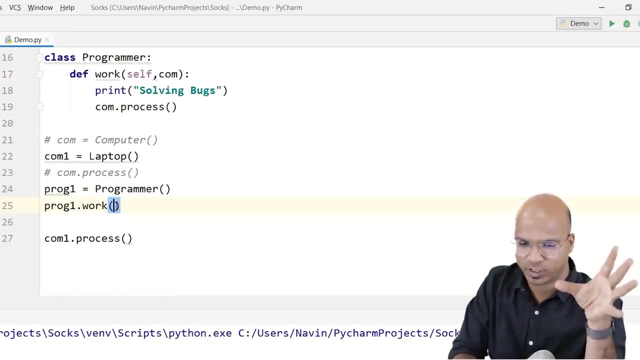 say it's writing. it's writing. okay, what's that okay? so now we got a whiteboard class as well, and the thing is this: whiteboard, can i simply pass an object of whiteboard here? see, in this work i have to pass an object of. if i pass the object of laptop, there's no problem. 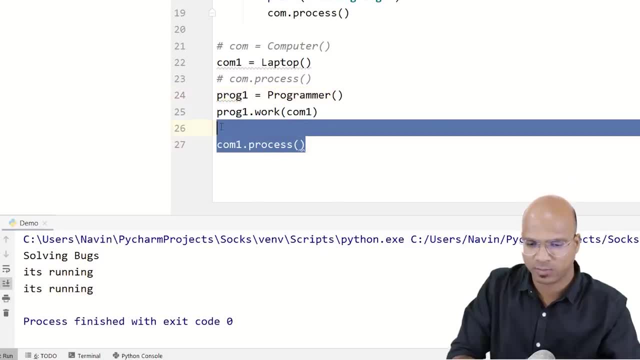 you can see if i run this code. and let me not call the process again, let me only call work. and if you say run this code, it works because it says solving bugs and it is running. so it is solving bugs because we are calling work, it is printing, it's running because from 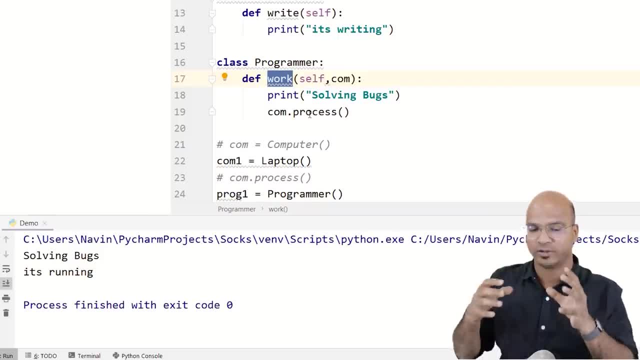 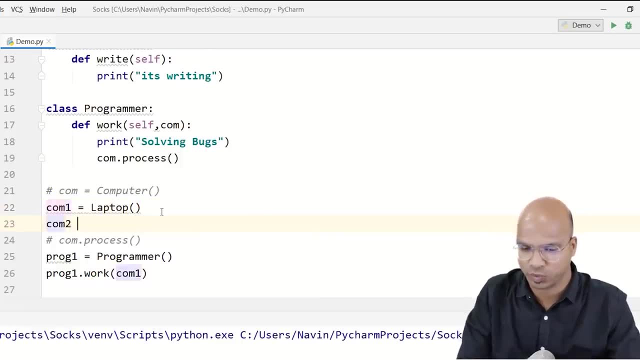 this method we are calling process, because as a programmer, we write a code and it you have to say process. right, but what if? if i create an object of a whiteboard, i will say com2 is equal to white board, and if i pass an object of whiteboard, you can see there's no compile time issue. i hope. 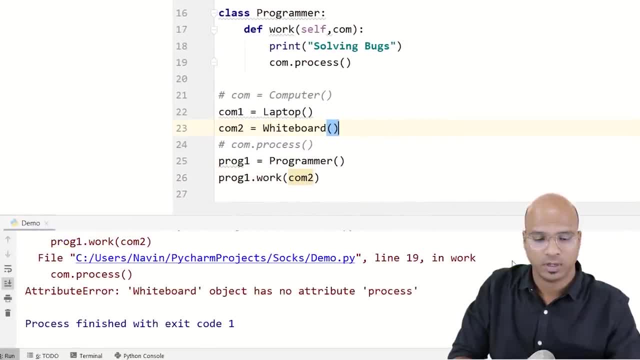 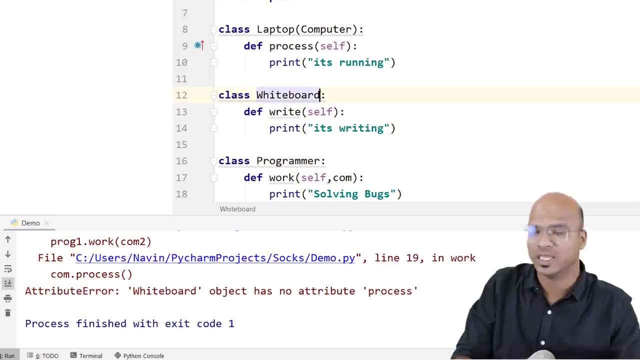 there is no compile time issue. but if i run this code you can see we got the issue because whiteboard don't have a method which is process. now why doesn't have a process method? because whiteboard, there's no compulsion for a whiteboard to implement or to have that method which is. 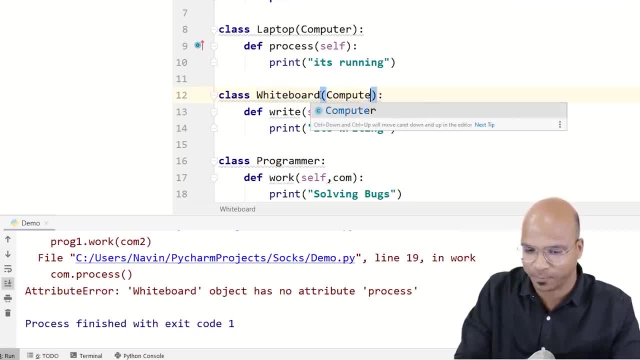 process right. and if you say, hey, whiteboard is a computer, in this case it becomes compulsion for a whiteboard to have this method, which is process. so that's the design aspect, right. it's not that you can't write a code without abstract classes, but then sometimes it's also depend upon the 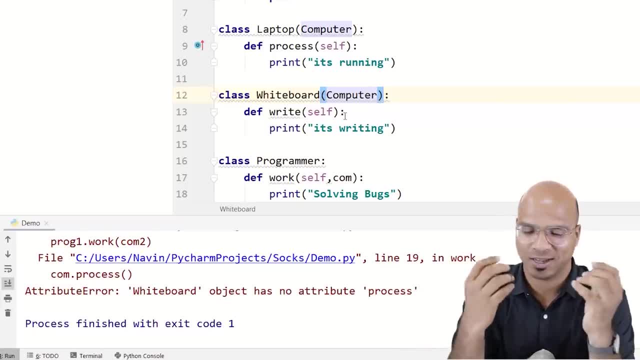 design, the way you design your application, the way you design your classes. so this is one way of defining a class. right, you can create abstract class so that the other classes will be will be having some signature or some restriction towards method to define, example, when you define apis. so